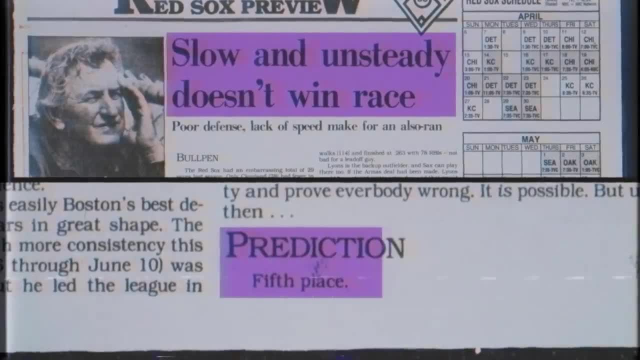 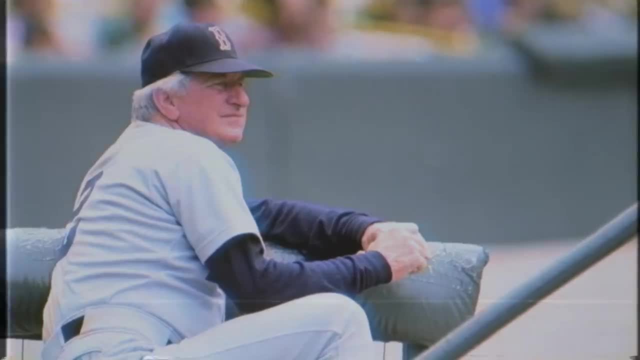 And the Red Sox came into the 86 season with critics doubting they'd even crack third place, something they hadn't done since 78, to say nothing of taking the pennant Last season under new skipper John McNamara. they finished in fifth place in the AL East, 18 and a half games behind Toronto. 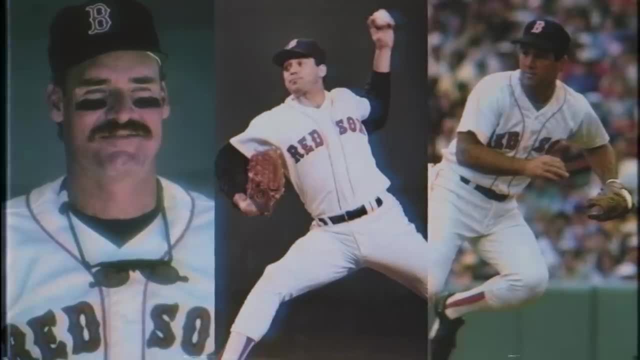 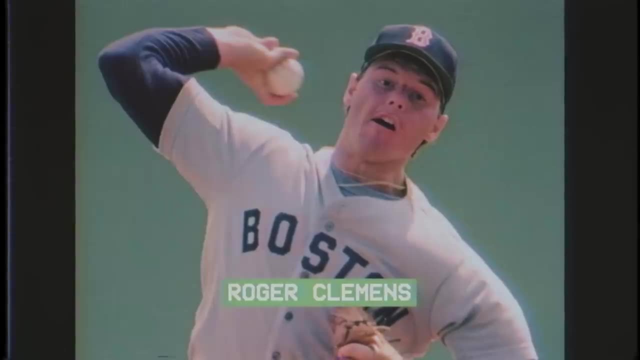 But the Sox have been spending the last few years building a core of powerful players. They brought up new talent like Wade Bonham, Bruce Boggs, Bruce Hurst, Marty Barrett and a hot young pitcher named Roger Clements, And this season, alongside veterans like Jim Rice and Dwight Evans, they've clicked. 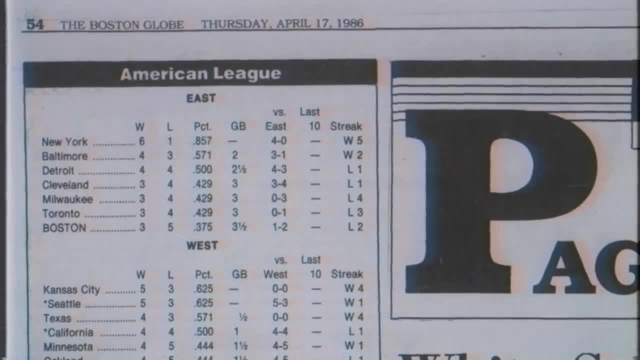 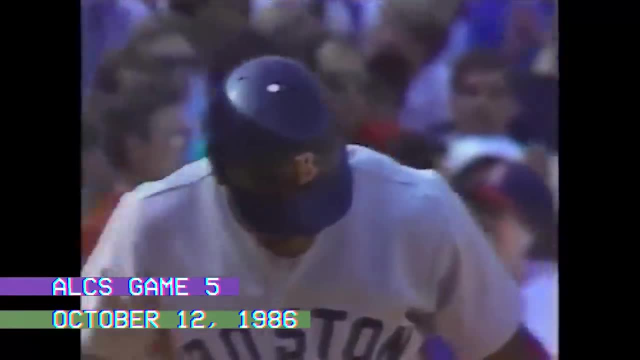 After a rough start in April that saw them at one point in dead last, the Sox rallied to finish May with a lead in the AL East that they never relinquished. They played an emotional ALCS, coming back from 3-1, which included a miraculous Game 5 performance by Dave Henderson. 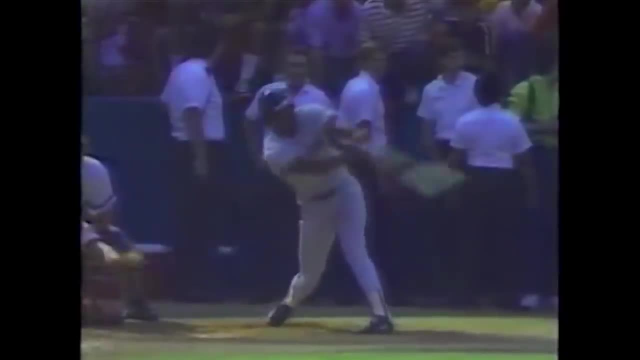 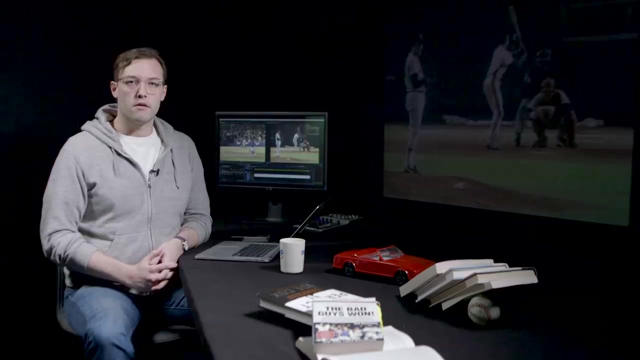 whose two-run homer in the ninth, with two outs and two strikes, saved the Red Sox from the brink of elimination. They came into this World Series ready to prove the haters and the losers wrong. And the 86 Mets came into this World Series as well, the 86 Mets. 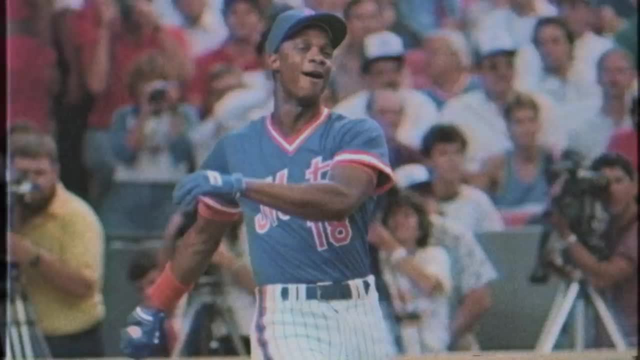 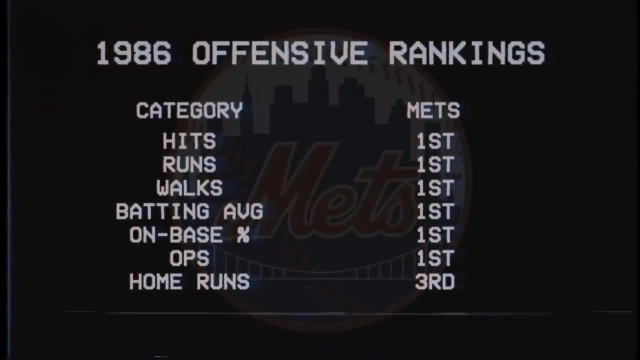 Keith Nails, Doc Straw, Mookie The Kid, A metric ton of booze and speed. The top spot in the National League in a bunch of offensive categories and third in home runs. The top record in baseball that year, with a franchise-best 108 wins. 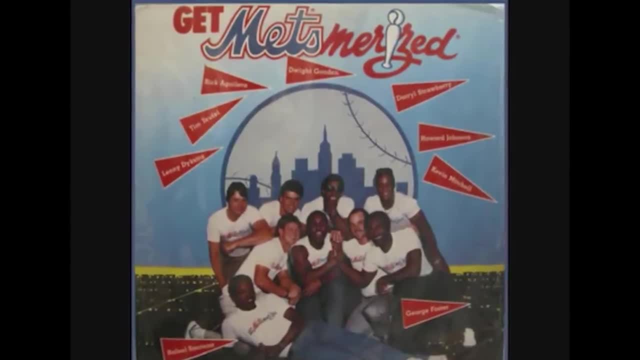 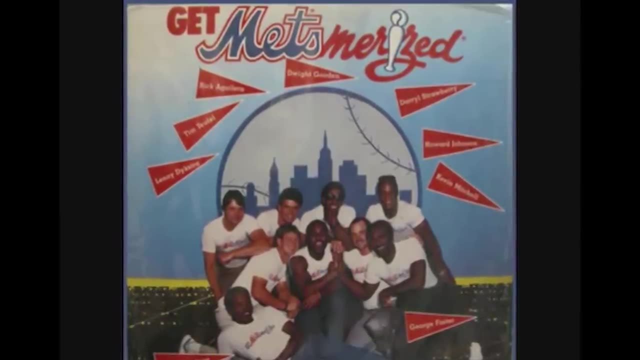 And, lest we forget, one of the most remarkable hip-hop stars in the world, One of the most remarkable hip-hop hits of the 80s. They recorded this in April, by the way, with a record of 1-0. 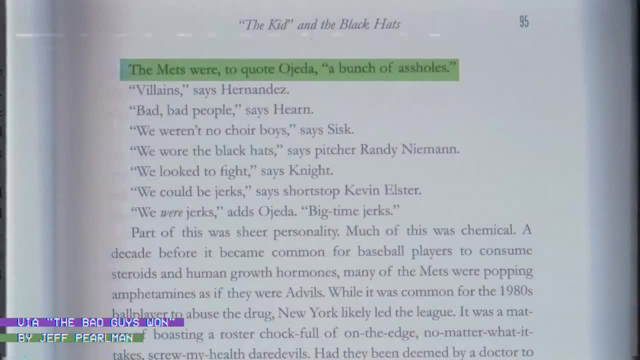 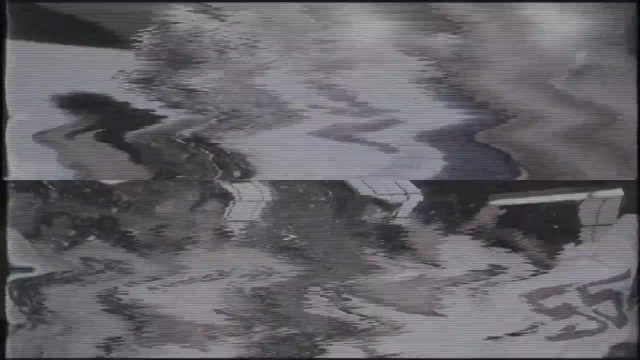 The 86 Mets have been a bunch of rowdy, cocky troublemakers with the dominance to back it up. But attitude and partying aside, they actually have some things in common with the Red Sox. They too have just come out of a dramatic championship series with a chip on their shoulder. 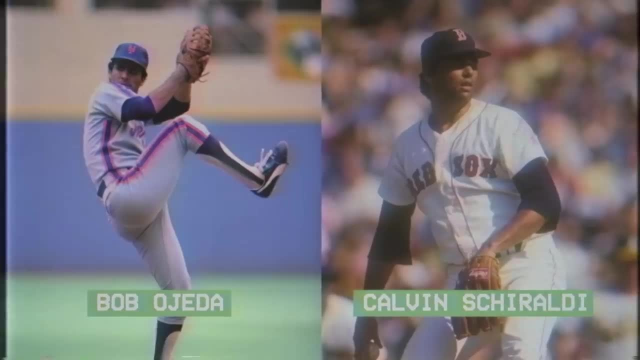 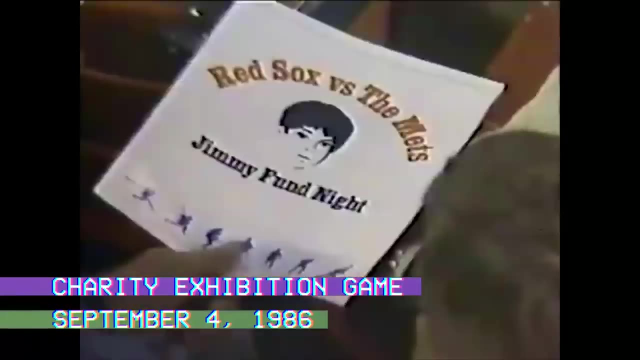 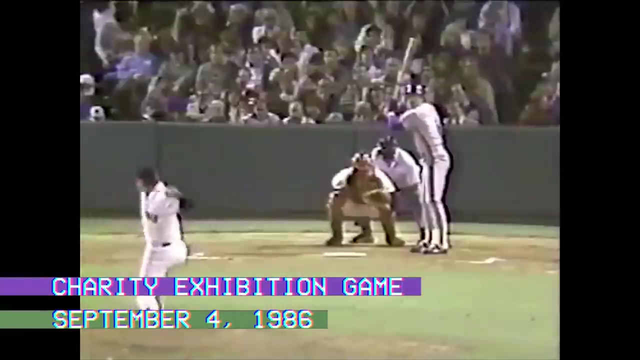 They, too, have just spent half a decade rebuilding. That included a trade between these two teams just this past offseason that swapped pitchers Bobby Ojeda and Calvin Chiraldi. In fact, although they're in different leagues, these teams even got to play each other once this season in a charity exhibition game on September 4th at Fenway. 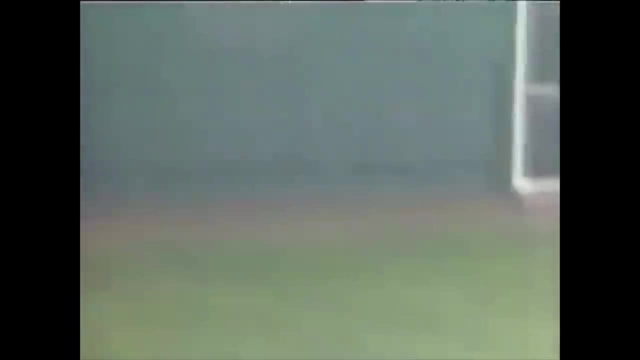 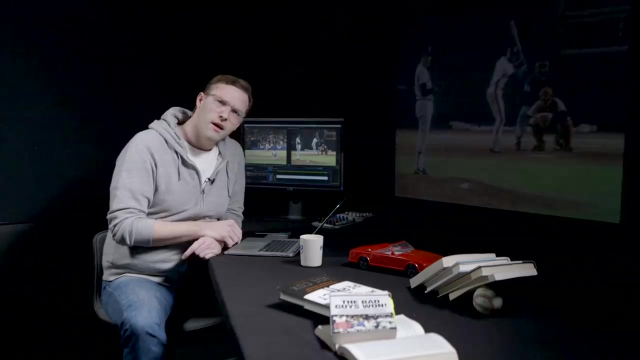 The Mets won that game 7-3,, a game in which Red Sox first baseman, Bill Buckner, let a ground ball slip right under his glove at first base, between his legs and into right field. Huh Anyway, the Mets came into the Fall Classic on fire. 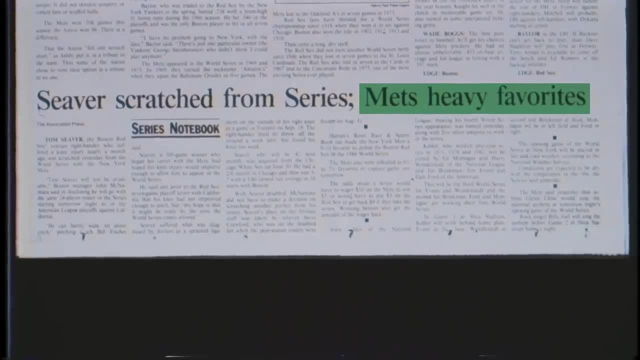 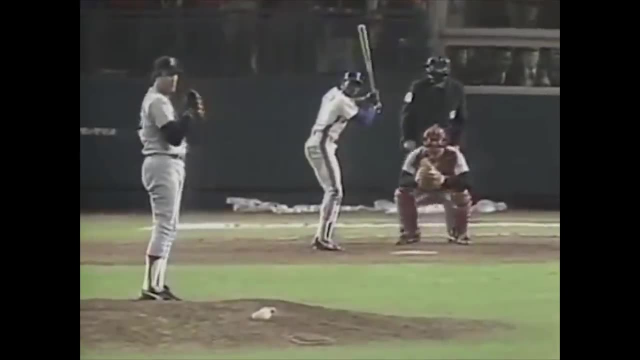 And the fact that they were favored to win out over Boston has turned up the heat even more for the Sox. But the fact that it's so close right now- tied in extra innings in Game 6, with two outs, a 3-2 count and a runner in scoring position- 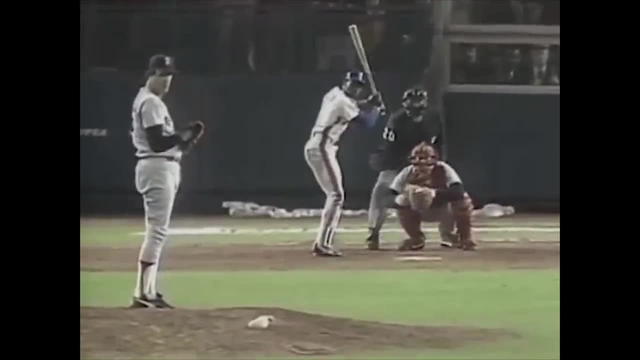 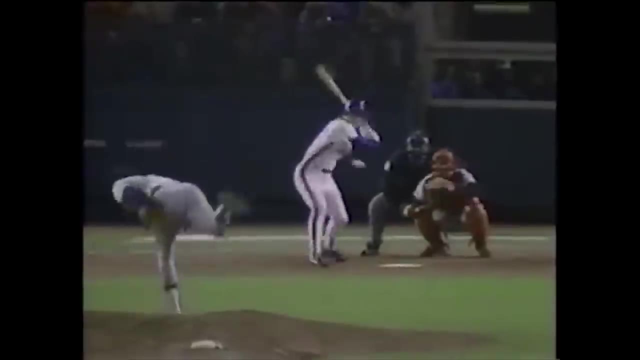 is a reflection on how these two teams have played this season and particularly how this series has gone thus far. Boston took Game 1 in a shutout at Shea thanks to Hurst and Chiraldi, but scored only one run off an error in the seventh from Mets second baseman Tim Tuffle. 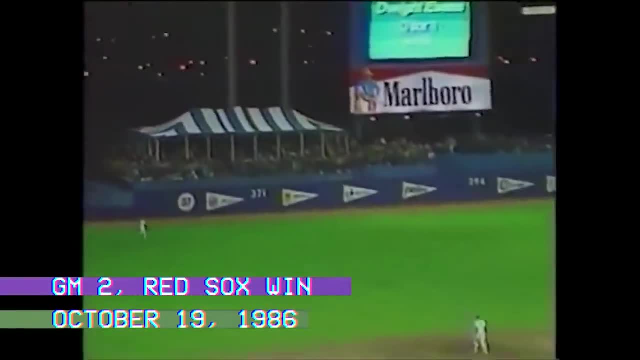 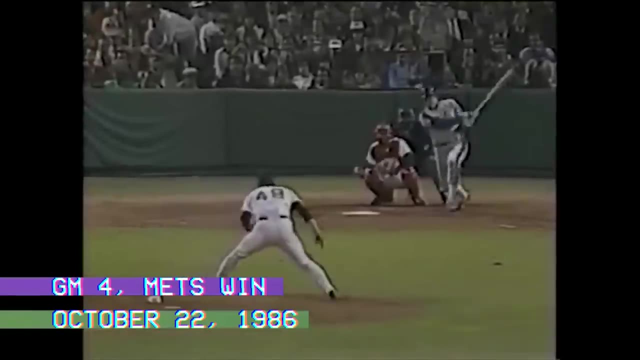 Boston's offense helped secure a commanding victory in Game 2.. But a leadoff homer in Fenway from Lenny Dykstra gave the Mets an edge they'd hold onto for all of Game 3, and in Game 4, Red Sox pitcher Al Knipper just got picked apart. 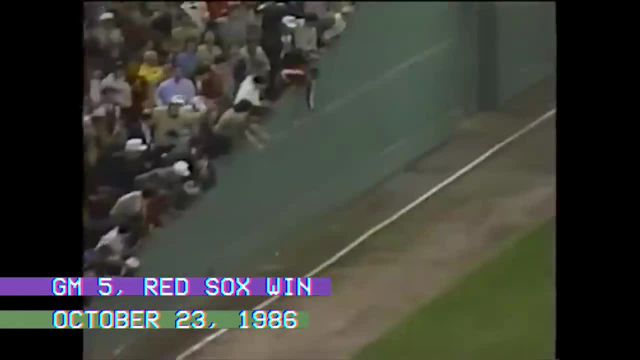 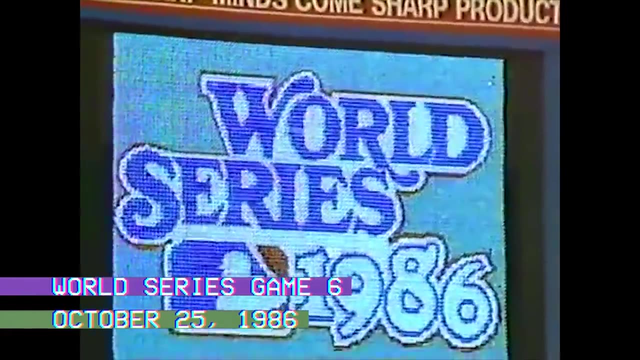 In Game 5, more heroics from Dave Henderson and Hurst gave the Sox the win and brought them back to New York, one win away from their first championship in 68 years. So these two teams have had dramatic swings all postseason, and tonight's game is no different. 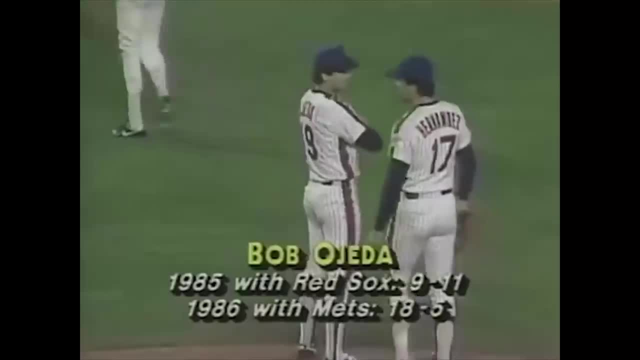 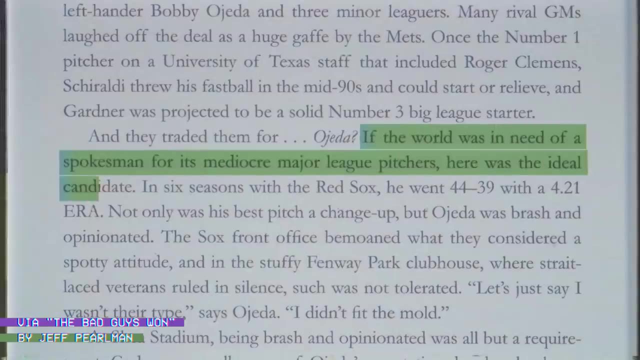 particularly when it comes to the pitching. The Mets started Bob Ojeda for Game 6, a left-handed pitcher they picked up in that offseason swap for Calvin Chiraldi. Though he didn't play great for Boston, he fit right in with the Mets and had a great season. 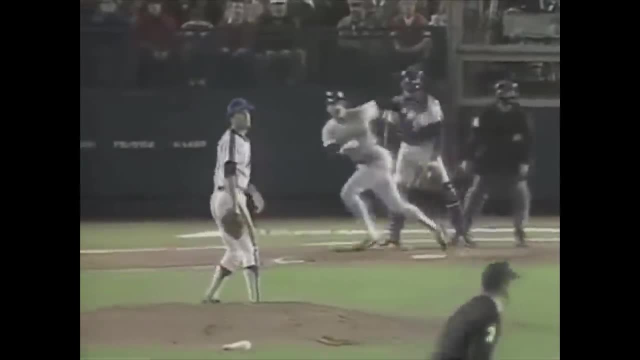 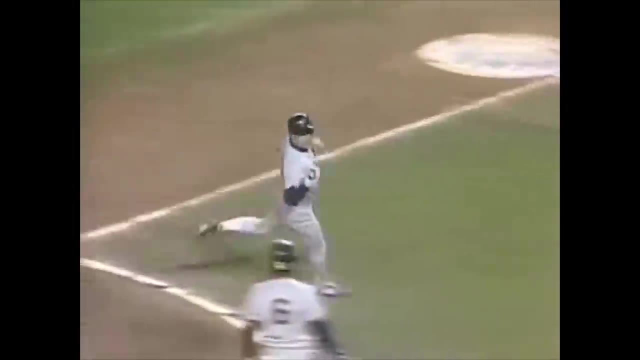 He pitched well in Game 3, but struggled a bit tonight in the beginning of Game 6, allowing a run in each of the first two innings, putting the Mets in an early 2-0 hole. The Red Sox started. Roger Clemens. 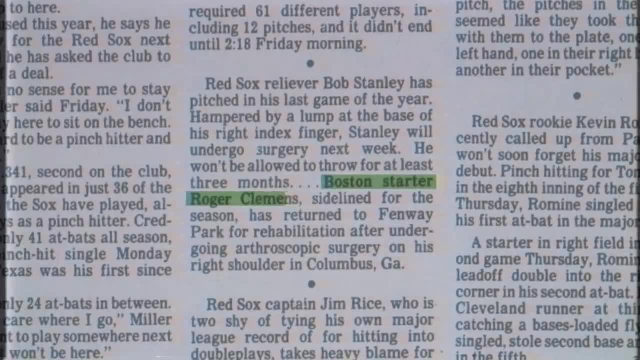 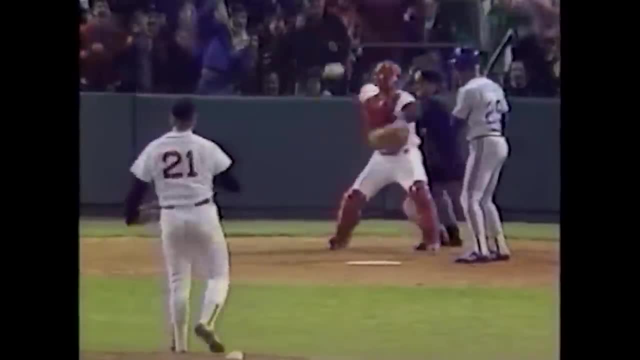 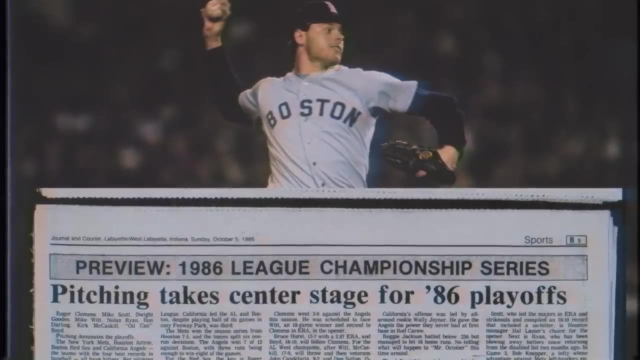 Clemens came into the 86th season as a bit of a question mark, having had surgery on his shoulder in the offseason. Clemens answered all questions in April when he made history by striking out 20 batters in one game. He followed up with an MVP-caliber season and is part of the reason Boston is in the World Series to begin with. 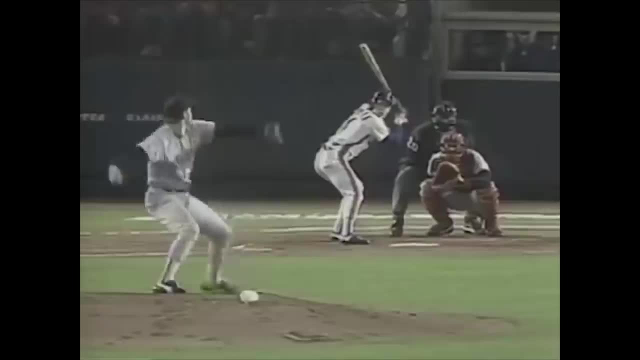 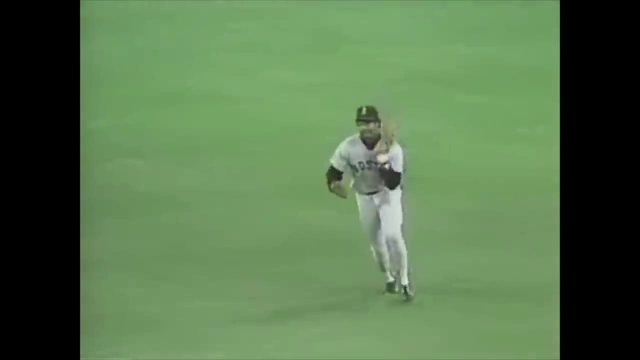 Tonight he's mostly kept the Mets at bay, holding them scoreless through the first four innings before giving up two runs in the bottom of the fifth and then pitching shutout innings in the sixth and seventh. But going into the eighth, skipper John McNamara pulled him and called out Calvin Chiraldi from the bullpen. 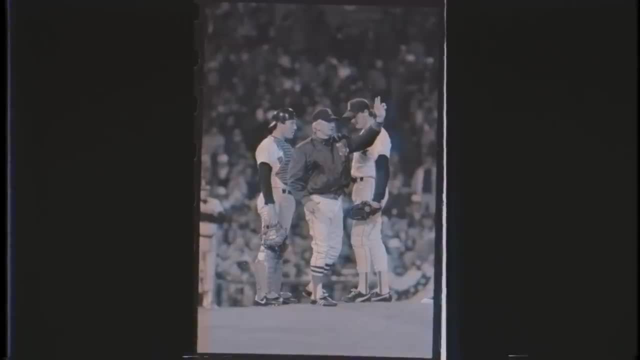 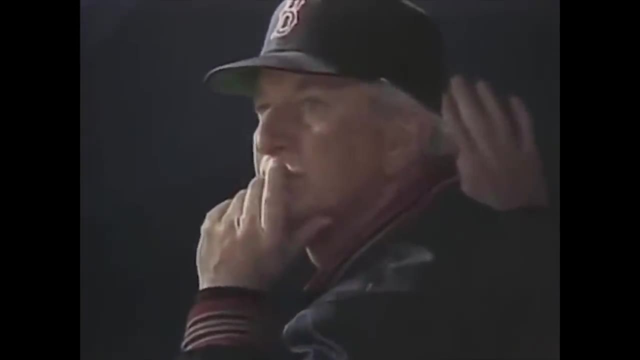 Why sit your star pitcher who's still rolling after seven strong innings? Maybe it was intuition, or maybe Clemens asked to be taken out of the game. In any case, McNamara's, confident in his closer Chiraldi's, proven himself a pretty solid relief pitcher for the Sox this season. 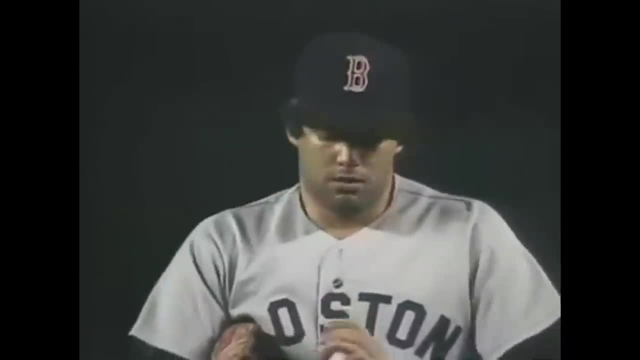 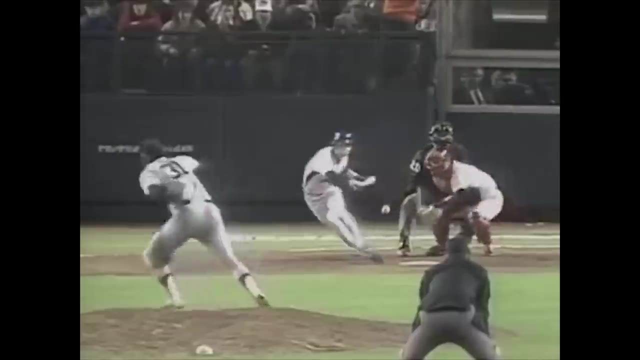 and Boston had a 3-2 lead going into the eighth. Chiraldi, however, had trouble against his former teammates as soon as he stepped up to the mound, After a single to Lee Mazzilli and a bunt from Lenny Dykstra. 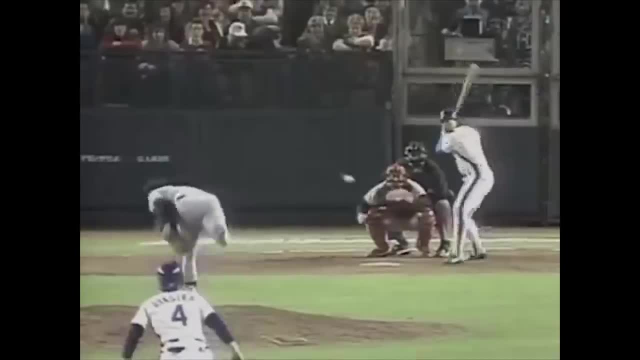 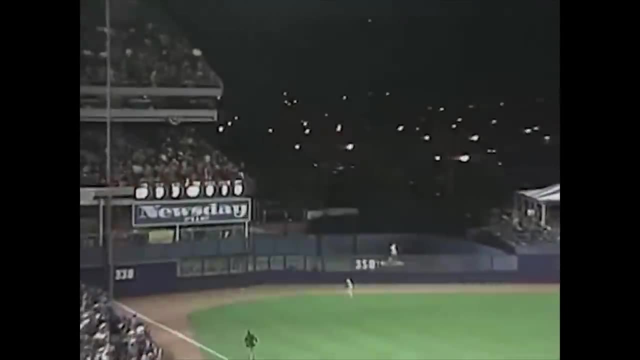 that Chiraldi failed to convert into an out. Gary Carter hit a sacrifice fly to bring in Mazzilli and tie the game at three, Fortunately for Chiraldi and for Boston. following a scoreless ninth, yet another miracle homer from Dave Henderson and an RBI single from Marty Barrett. 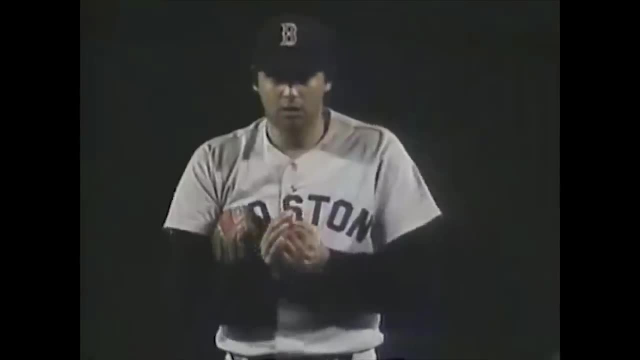 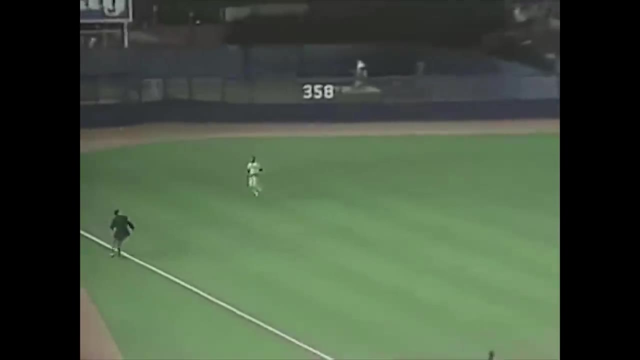 would bring the Red Sox lead back to 5-3.. Chiraldi came back to the mound needing just three outs to end it once and for all, And for a moment he looked like he was going to win. He looked like he would do just that. 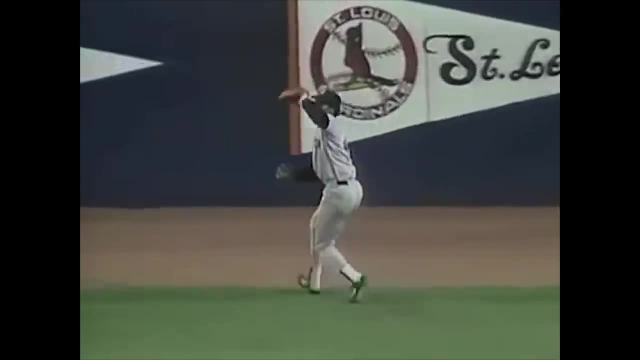 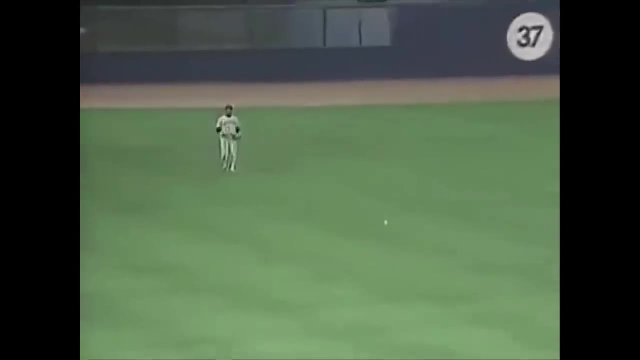 getting fly ball outs from Wally Backman and Keith Hernandez, But then with one out between him and history disaster. A single from Gary Carter, Another single from Kevin Mitchell and then a line drive from Ray Knight to right center that scored Carter. 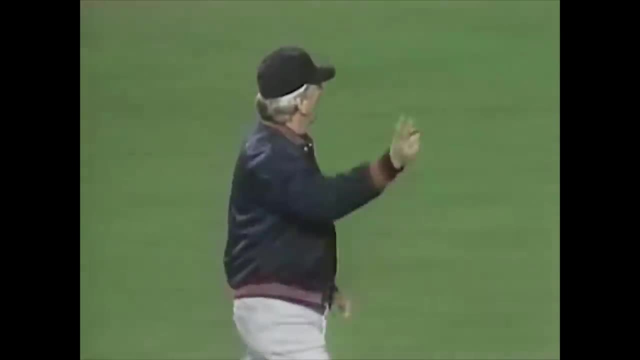 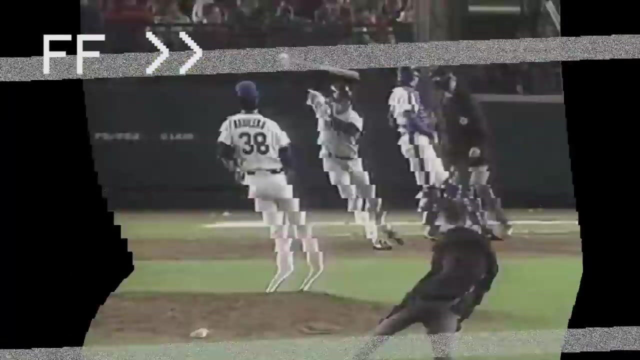 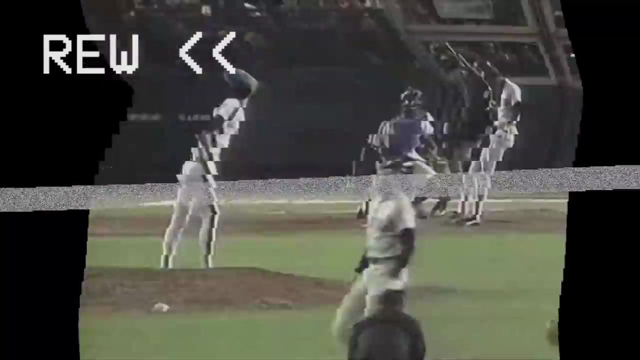 and sent Mitchell the tying run to third base McNamara, trying to stem the bleeding, called the Red Sox of ten years, Bob Stanley, to the mound to face the batter who now stands at the plate, Mookie Wilson. But first Bob Stanley had to contend with a greater foil himself. 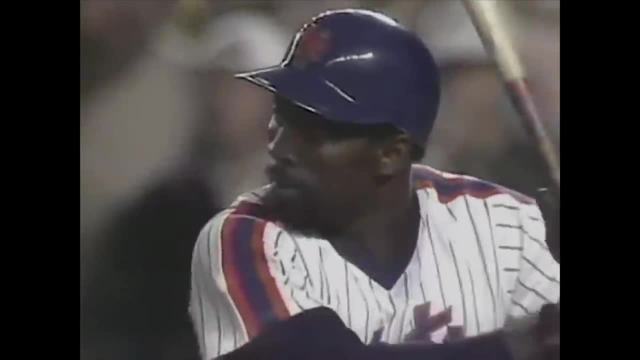 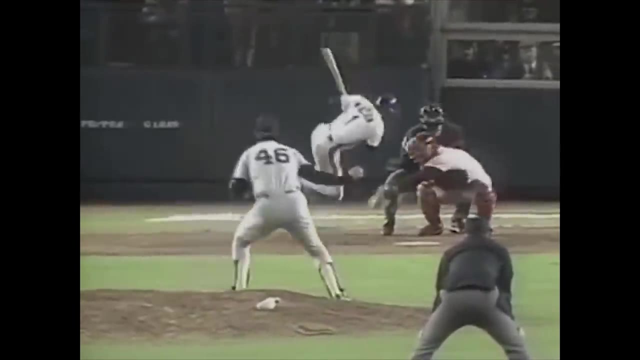 After six pitches, Stanley got the count to 2-2.. The Sox are again one strike away from victory. On his seventh pitch of this at-bat, Stanley threw a wild one way inside, sending his catcher to the backstop to retrieve it and allowing Mitchell to score. 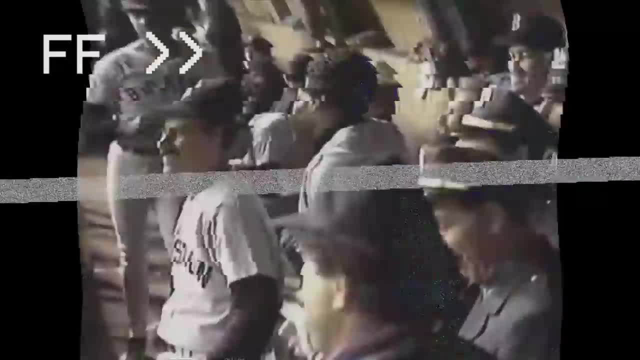 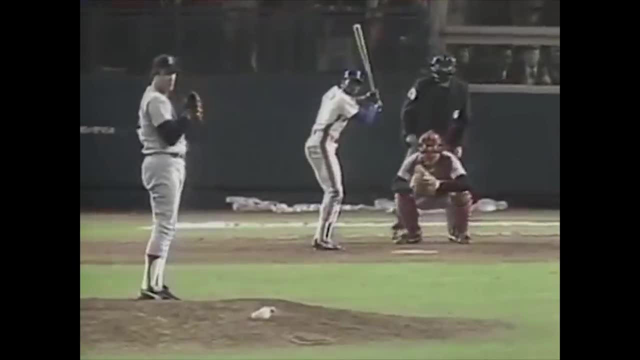 tying the game and moving Ray Knight the winning run to second. And now suddenly all the Mets need is Mookie Wilson to bring him home. And it's kind of a miracle Mookie Wilson is standing at the plate right now. In March, during a preseason drill, 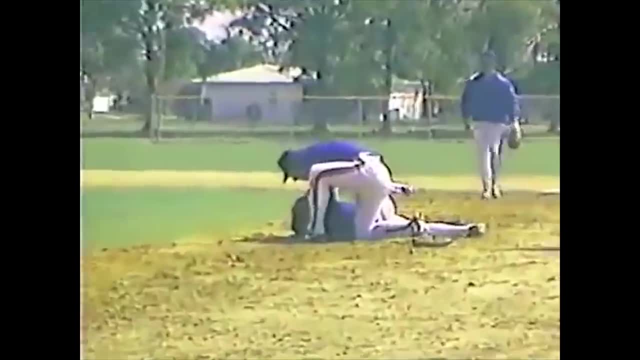 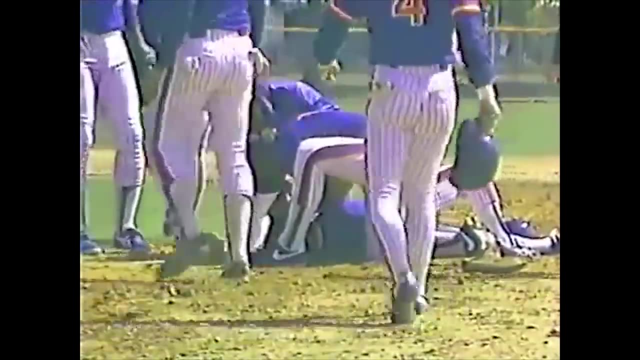 Mookie suffered a pretty severe eye injury when he took an errant ball to the face. that shattered his sunglasses and very nearly blinded him. Did it break the glass? Did it break the glass? Oh God it did. Luckily, Mookie, a Mets fan favorite. 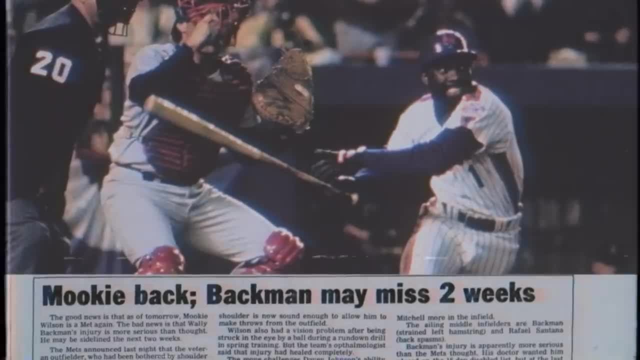 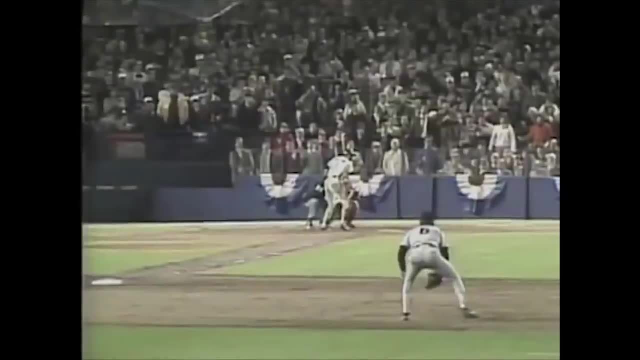 was able to recover and was back in the starting lineup by May. Good thing too. he's one of the Mets' best batters and one of the fastest guys in the league, something that Buckner at first base is well aware of. 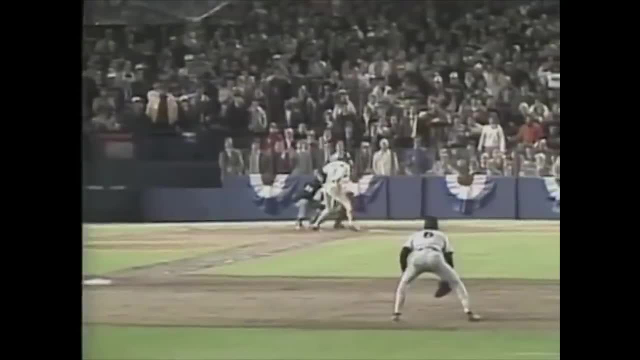 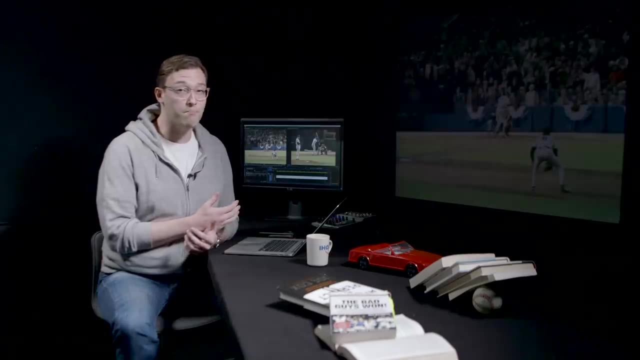 He knows he'll have to hustle to beat Wilson to the bag if it comes to that. Okay, let's talk about this guy at first, this Bill Buckner. Going into Saturday there were questions as to whether or not he should even be in the game. 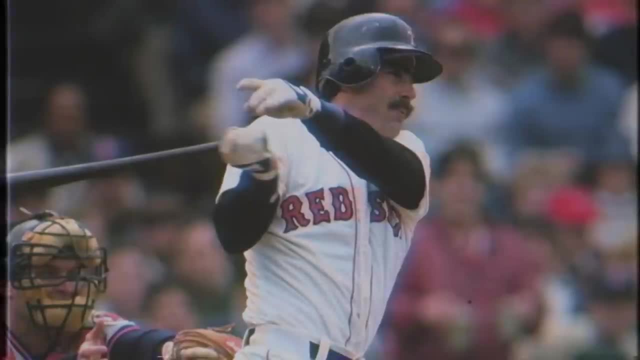 but not because of his fielding. Here's something that might surprise you: Bill Buckner is a good baseball player. In fact he's a borderline Hall of Famer. He's a veteran workhorse, a certified slugger, a former NL batting champion. 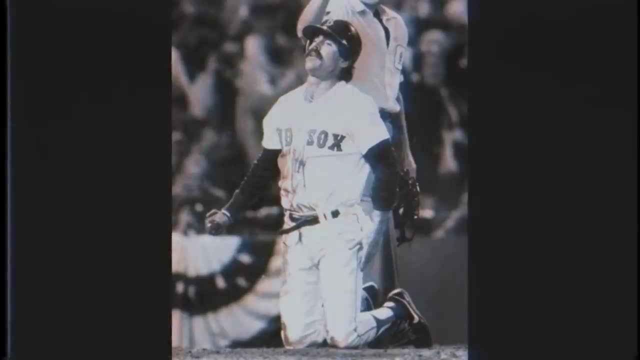 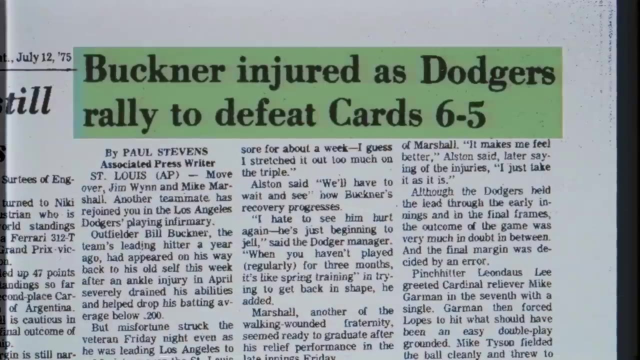 and All-Star who has a history of coming through in the clutch. But Buckner is banged up Badly. He's got famously bad knees and ankles and in 1975, suffered an Achilles injury that's been plaguing him for over a decade. 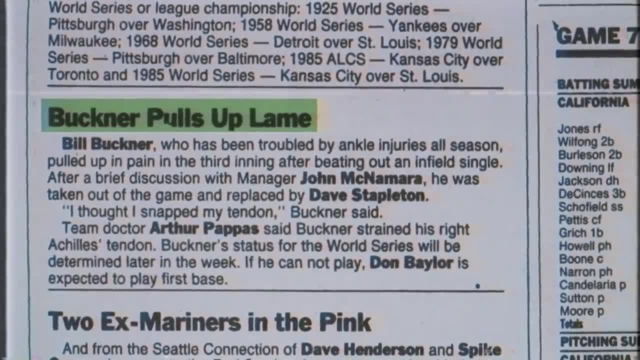 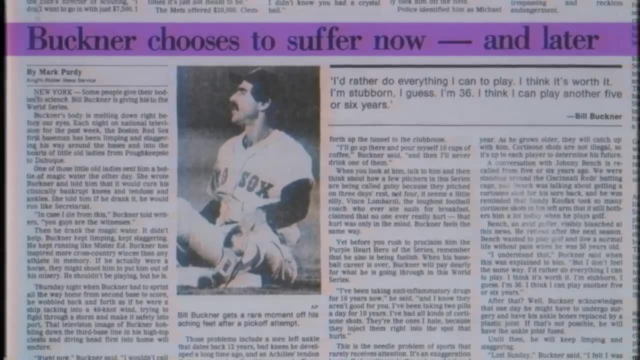 Just a few weeks ago, in Game 7 of the ALCS, Buckner hurt himself so badly he thought he had snapped his tendon. Now, in the final games of this World Series, he's in agony. He spends hours after games icing himself. 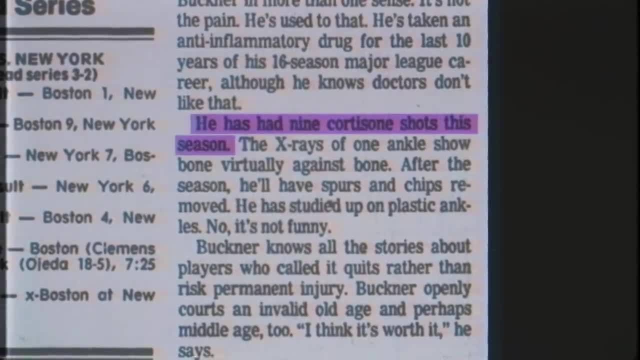 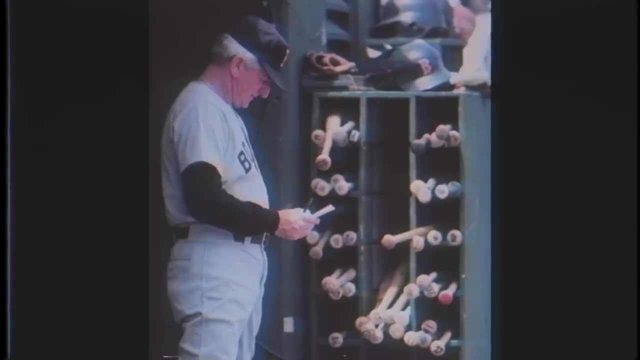 He's had nine cortisone shots this season alone and x-rays have shown that one ankle is basically bone against bone. So, going into Saturday's game, some wondered if it was worth it for John McNamara to start a first baseman with mobility problems. 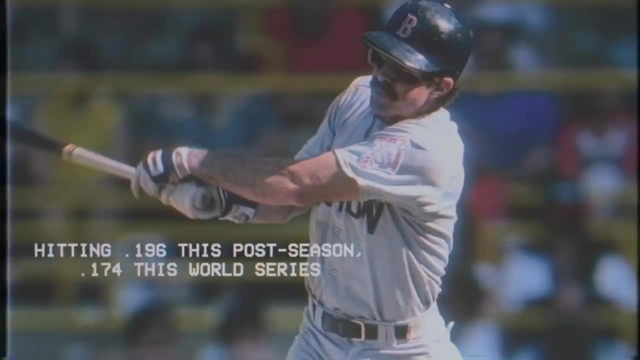 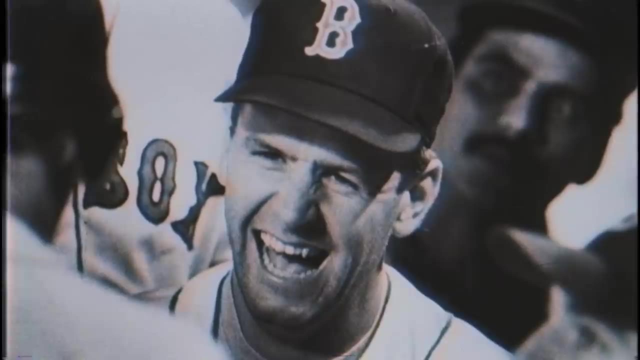 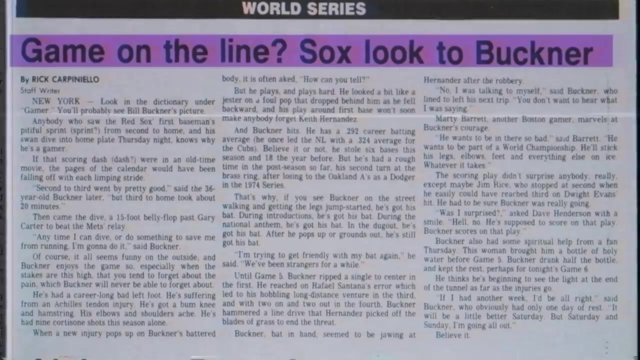 especially given the fact that this postseason he hasn't been at his best, at least offensively. Why not sub in defensive replacement Dave Stapleton- which he's done late in games plenty of times all season- Because, simply put, there was pretty much no way Bill Buckner was going to sit in the Boston dugout at 36 years old?